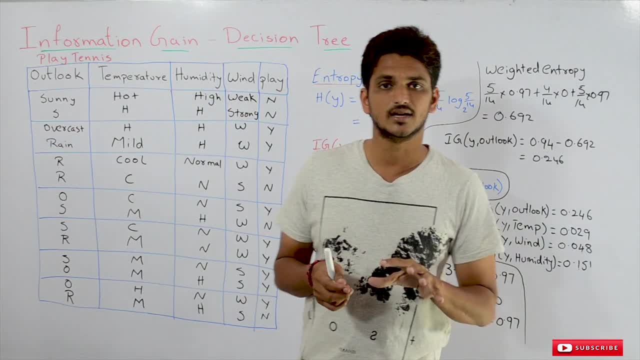 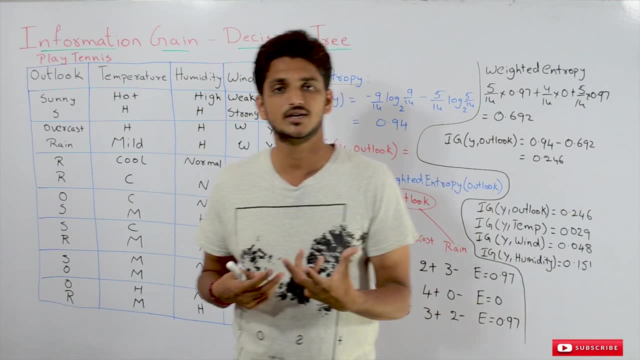 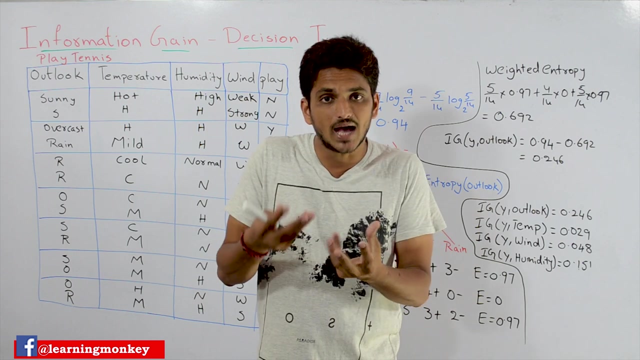 And in our graphical intuition class we already discussed that. the goal of decision tree? Suppose, let us say in our example data set, if you are having 10 columns, what is the goal of decision tree? Identify a column that gives the best separation means that the column that is helping us a lot in doing the best prediction. 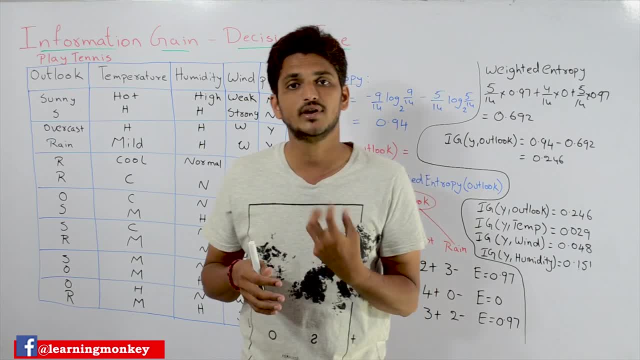 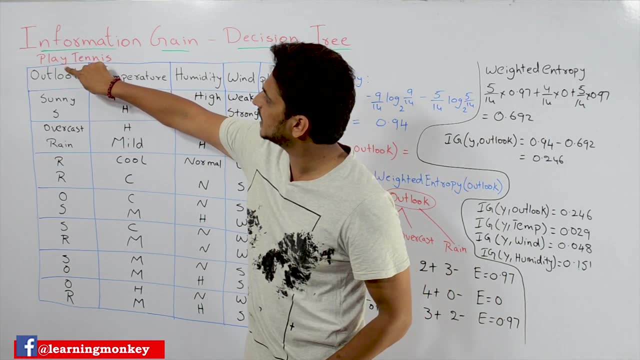 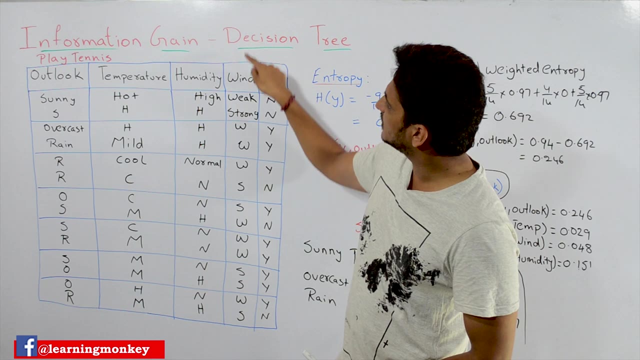 That column has to be identified. How to identify that column? Using information gain. So what we do here is: we will calculate information gain for outlook, We will calculate information gain for temperature, We will calculate information gain for humidity. So we will calculate information gain for wind. 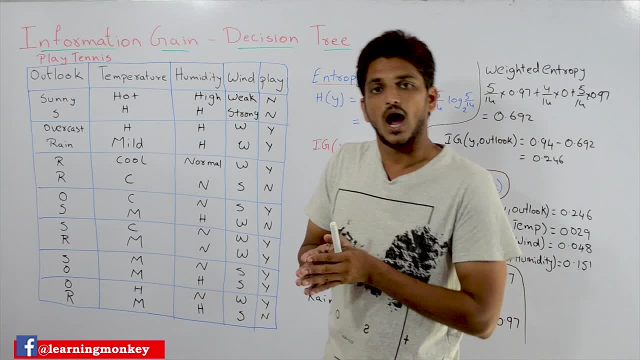 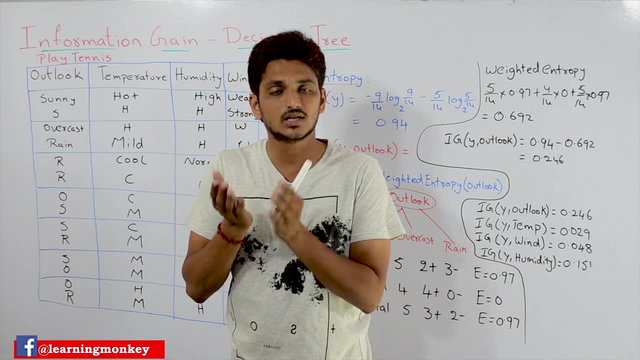 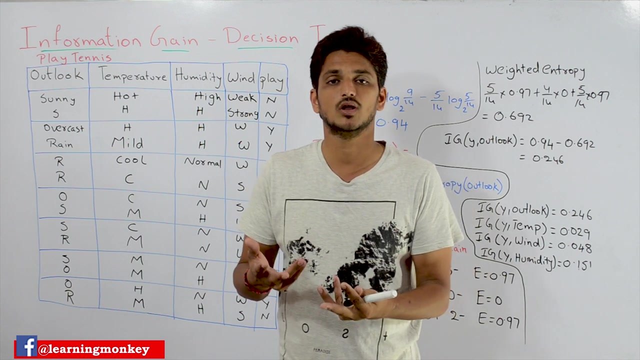 For all the columns We will calculate information gain And out of these four columns, which column is having the highest information gain value? That column will be taken into consideration. That column is taken as the best column, So why that is best column? 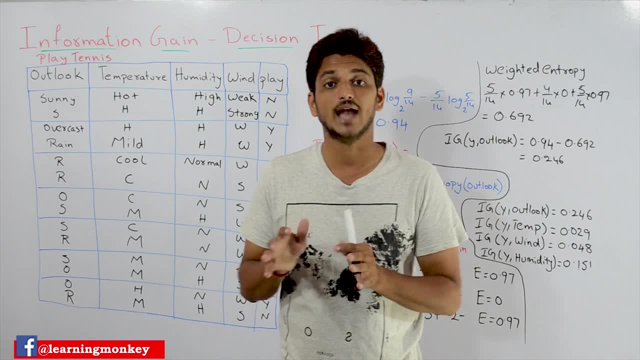 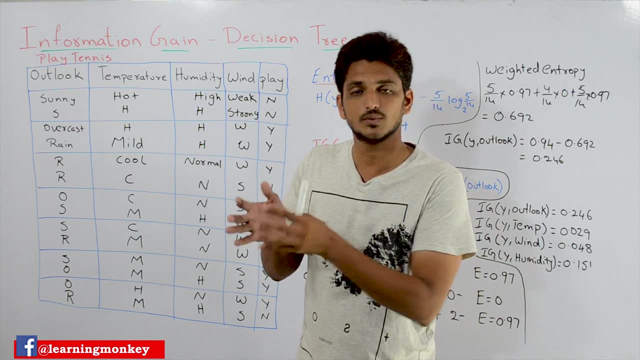 First, we will understand how to calculate information gain. At the end of the class we will discuss why highest information gain value column is taken as the best column. That concept we will understand at the end of the class. So coming to how to calculate information gain. 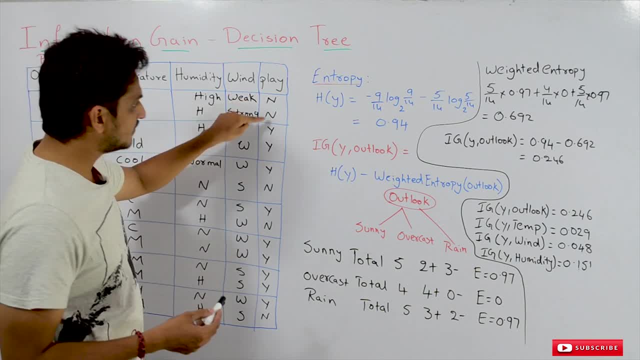 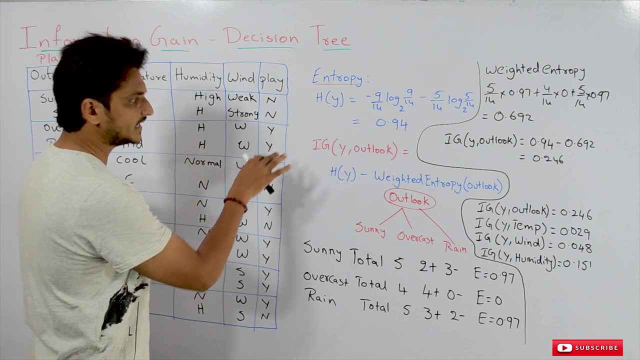 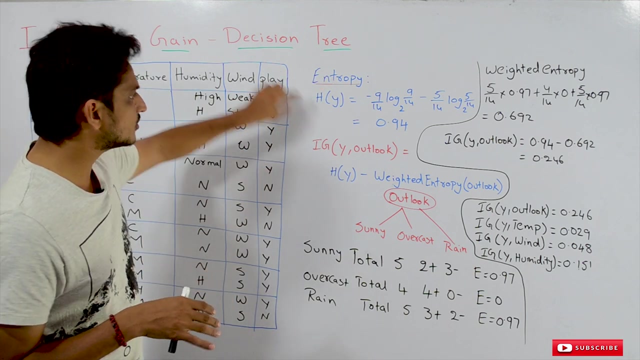 This is our data set. In this data set we are having 5 negative points, 9 positive points. Positive points means s means play tennis, n means they do not play tennis. negative points: And in our last class we discussed that- how to calculate entropy for this data set. 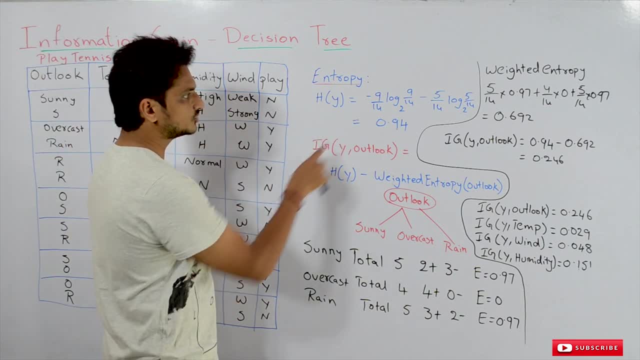 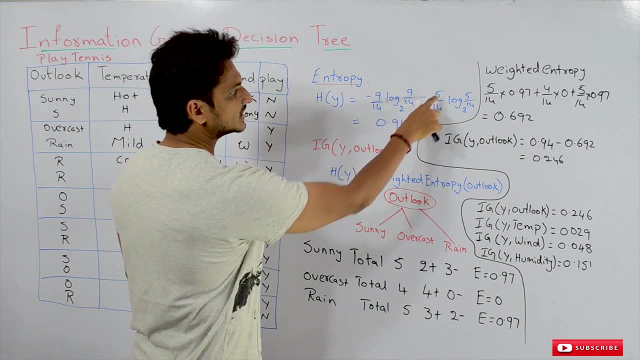 h of y is equal to 9 positive points. 9 out of 14 points, 9 are positive points: 9 by 14 minus 9.. 9 by 14 minus 9 by 14 log 9 by 14 base 2 minus 5 by 14 log 5 by 14 base 2.. 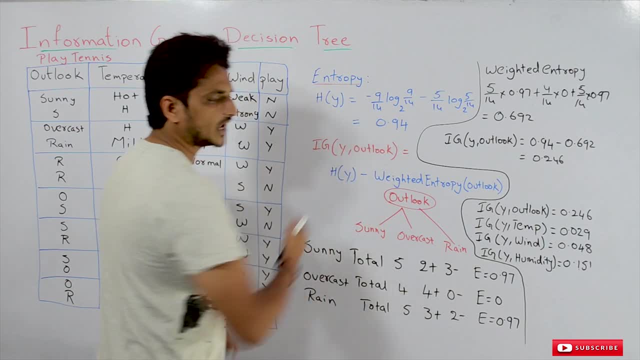 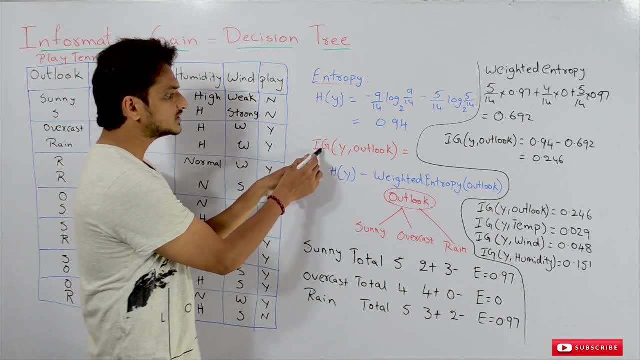 So if you calculated it, the entropy value, we got it as 0.94.. So this is how we calculate entropy value, How to calculate information gain value. Information gain for y comma outlook. So we are calculating information gain for outlook now. 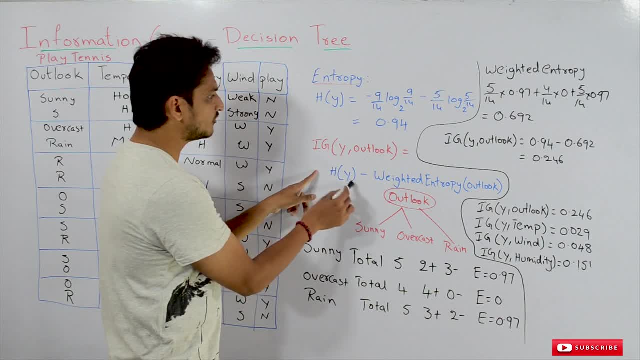 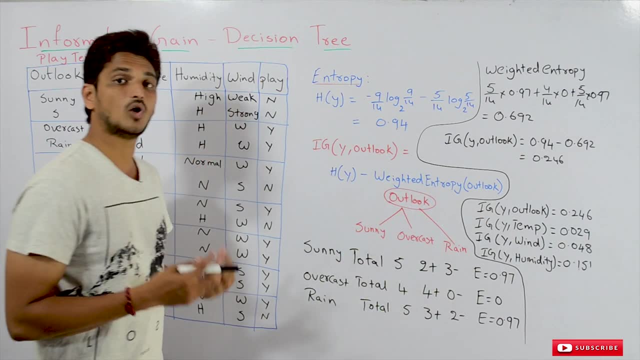 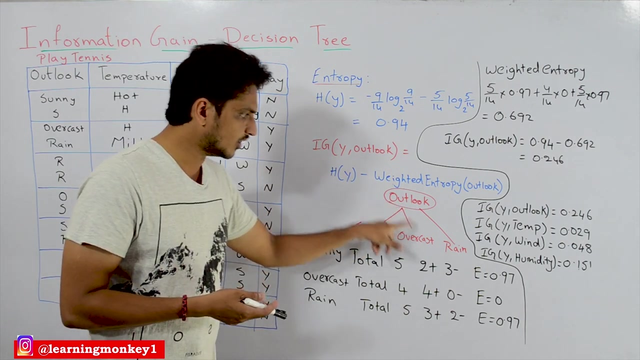 So how we calculate this is equation: is h of y means the data set, entropy value minus Weighted entropy of outlook. So how to calculate the weighted entropy of outlook? So in outlook, how many separations we have. We are having sunny, overcast and rain. 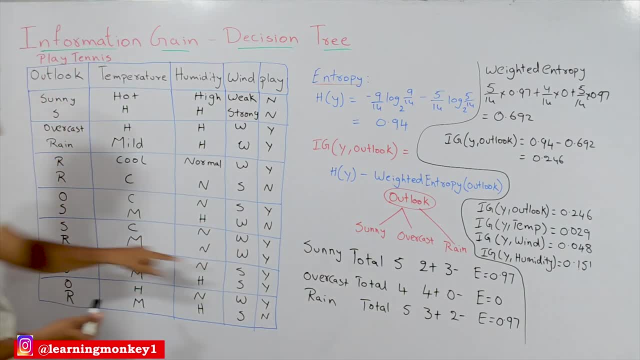 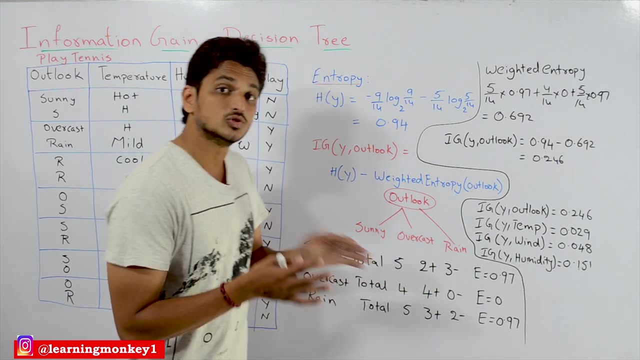 In this. how many sunny data points are there? We are having sunny total 5 data points. Out of that we are having 2 positive and 3 negative points. So calculate entropy only for sunny. So 2 positive and 3 negative values. 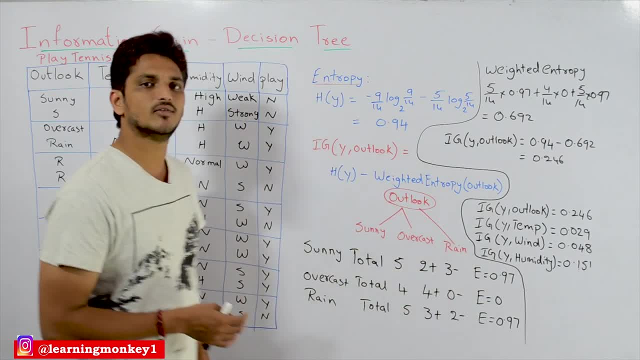 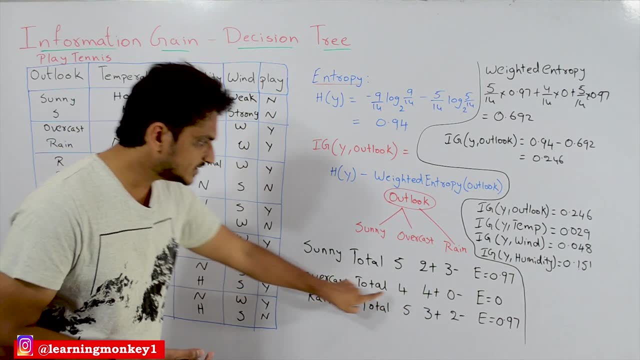 So E is equal to 0.97.. So you do the calculation: E is equal to entropy is equal to 0.97.. The same way, overcast is having 4 data points. Out of this 4 data points, all are positive points, 0 negative points. 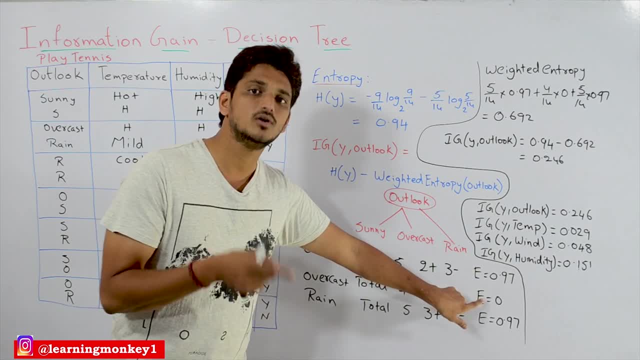 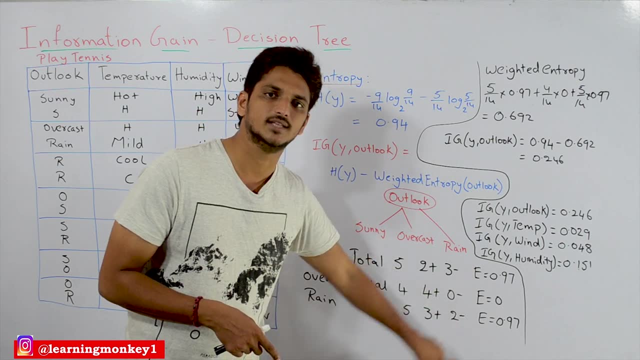 So if all are positive points, what is the entropy value? 0.. The same way, rain: total 5 points, 3 positive and 2 negative points. Entropy is equal to 0.97.. So we calculated entropies for sunny. 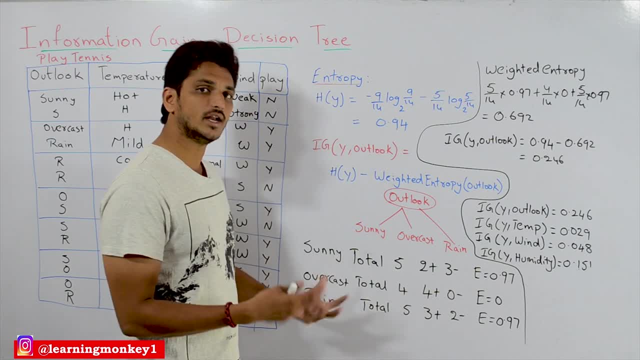 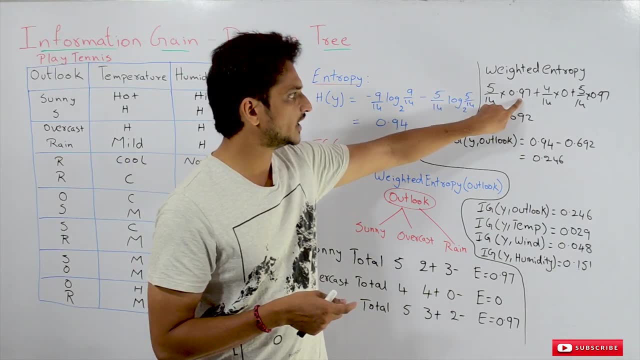 For sunny, overcast and rain. So how to calculate the weighted entropy, Sunny, how many points are there? 5 out of 14.. So 5 by 14 into 0.97, the entropy value Plus 4 by 14, entropy is equal to 0. 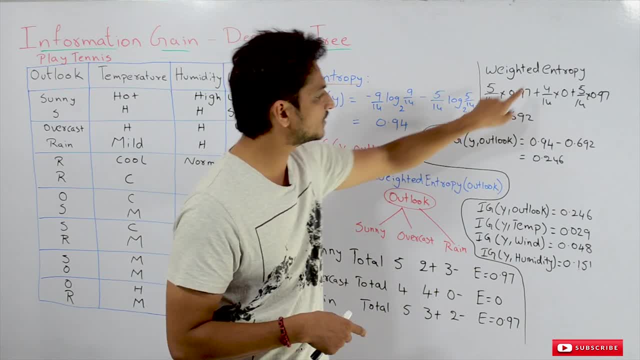 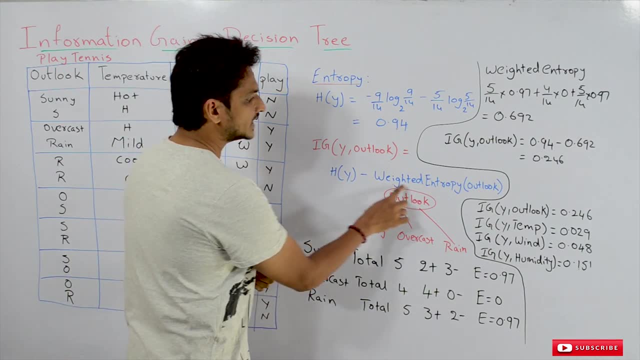 Plus 5 by 14 into 0.97.. The total weighted entropy we got here is 0.692.. So what is the equation for information gain? h minus weighted entropy of outlook. So h is 0.94 minus 0.692.. 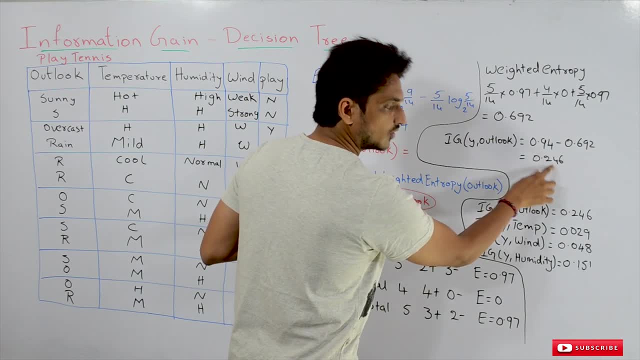 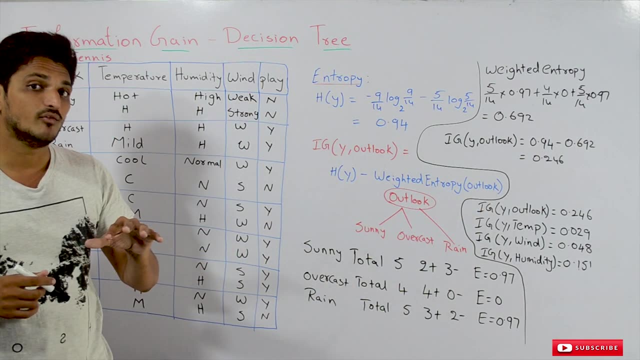 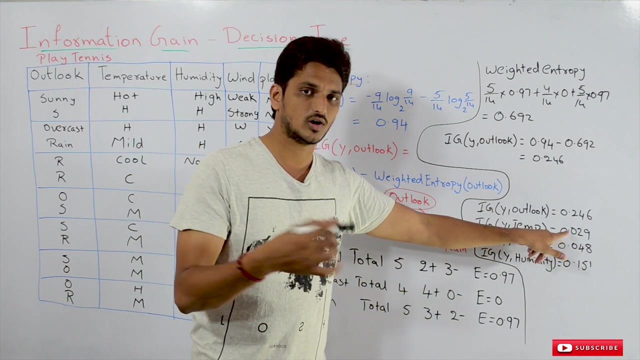 We got it as 0.246.. So information gain value for outlook column is equal to 0.246.. The same way we have to calculate information gain for temperature: 0.029.. You do the calculation. We are not doing calculation here. 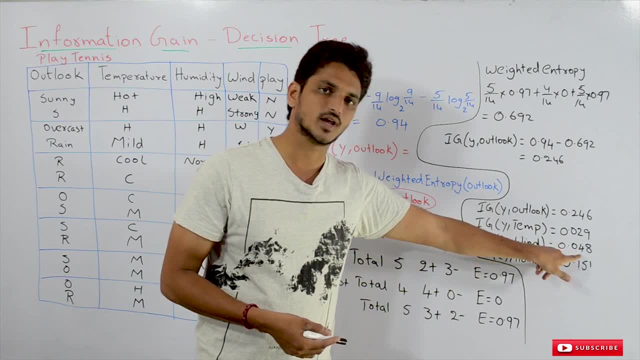 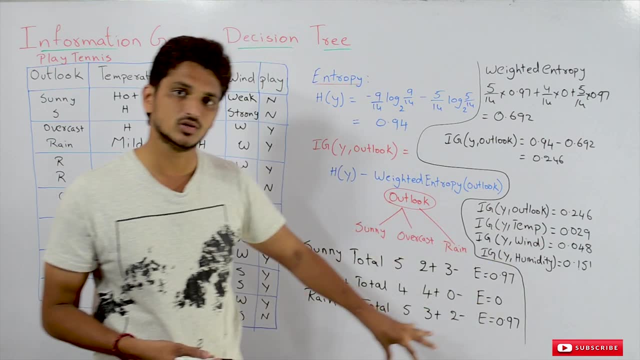 Information gain for wind: we got it as 0.048.. Information gain for humidity is equal to 0.151.. Out of these 4 columns information gain values, which one is having the highest information gain value? Outlook is having the highest information gain value. 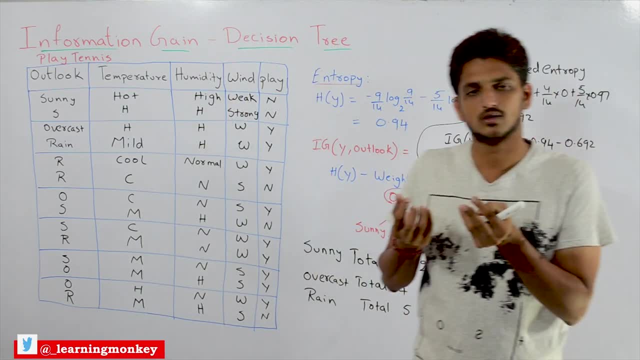 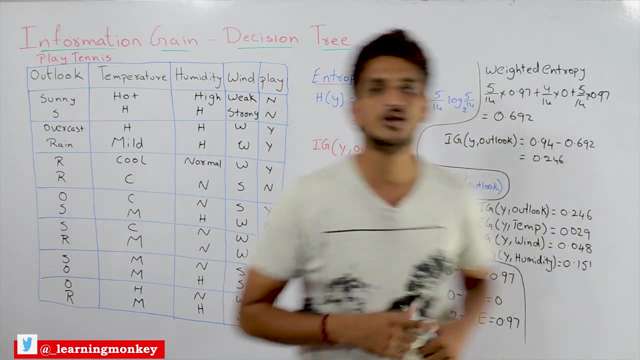 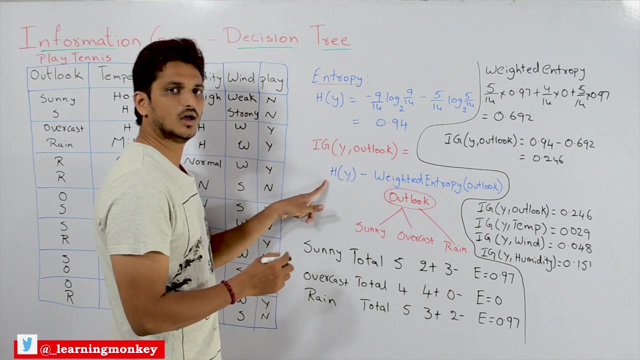 So we pick outlook as the root node. So why? So? why highest information gain value is taken as the best column. Let us understand with the equation. So what is the equation here? h minus weighted entropy of outlook. h minus weighted entropy of temperature. 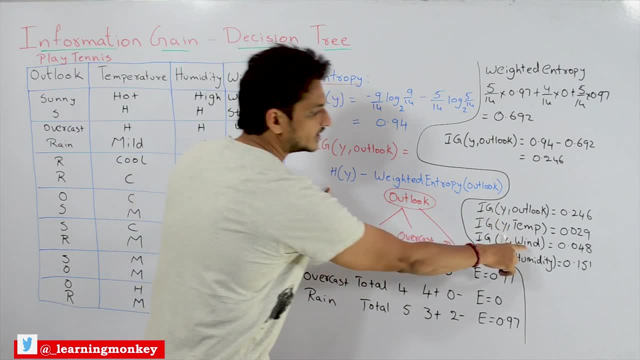 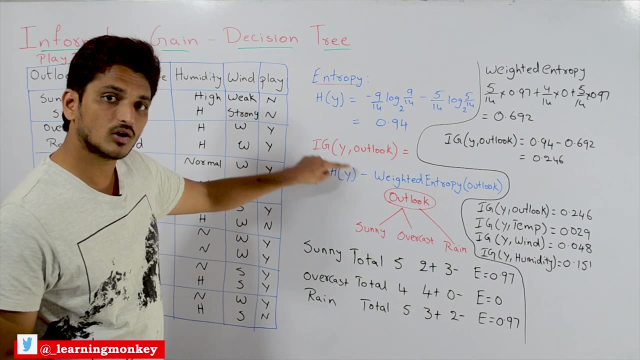 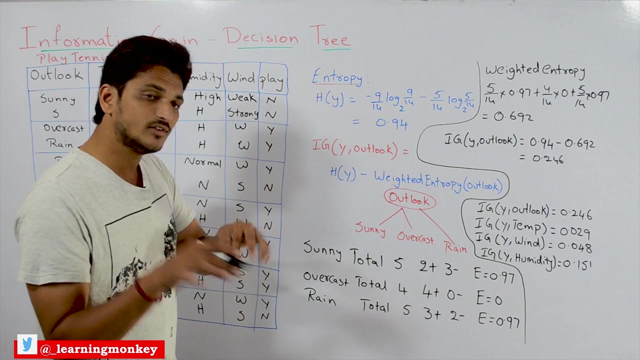 h minus weighted entropy of wind, h minus weighted entropy of humidity. So h is common for all the columns. What is changing here? Weighted entropy of outlook. Weighted entropy of temperature. So when the information gain will be maximum, When this value will be maximum. 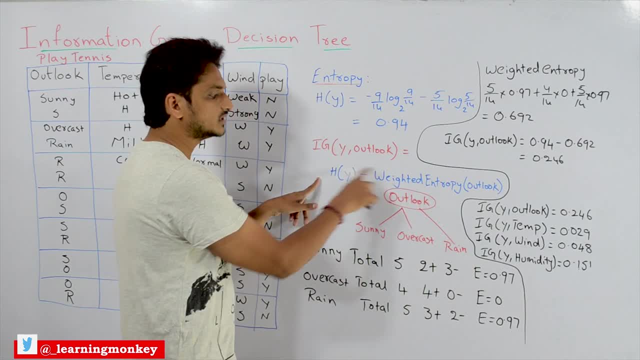 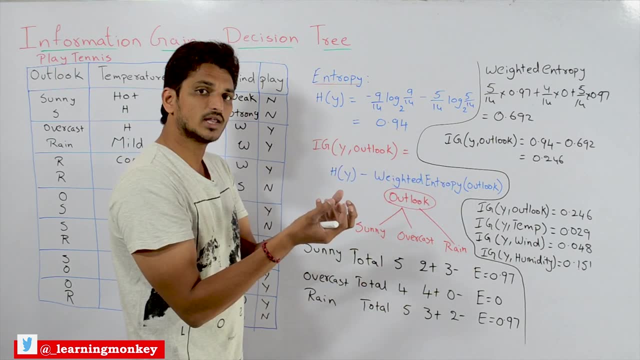 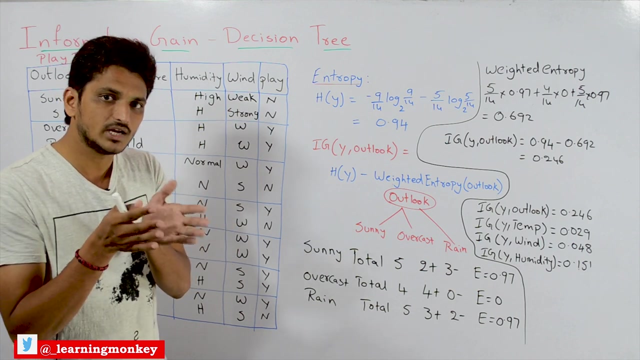 If weighted entropy value is minimum, because we are doing subtraction from h. So when weighted entropy value of outlook is minimum, then we are having information gain value maximum. So when weighted entropy of outlook value will be minimum, When the weighted entropy value will be minimum, 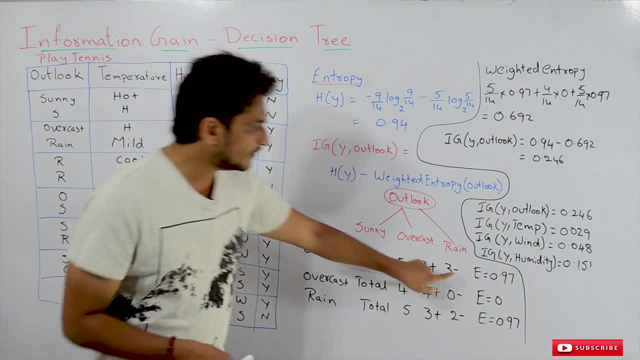 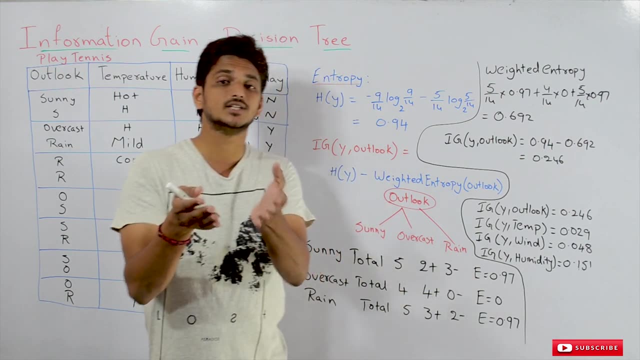 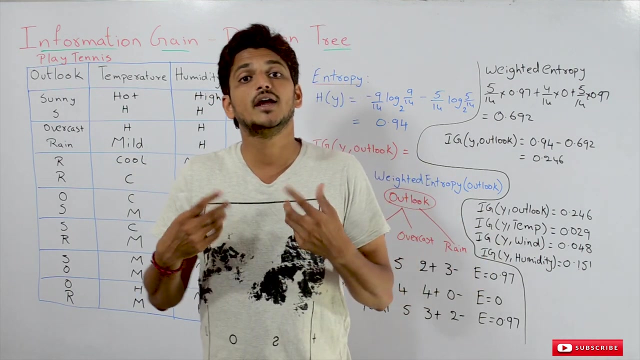 Let us check it So: weighted entropy value will be minimum when entropy values of the divisions are minimum. So that is what we discussed in our last class in entropy class. If entropy value is minimum, what we have discussed- We are very certain to do prediction. 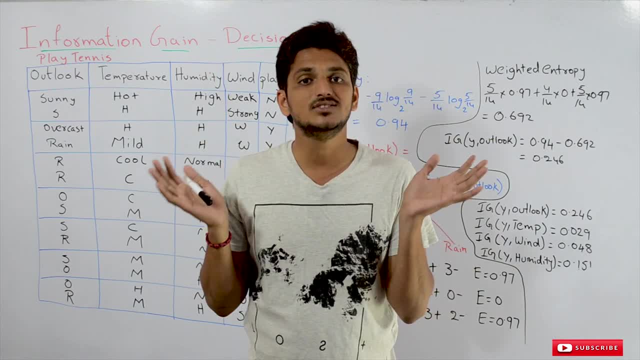 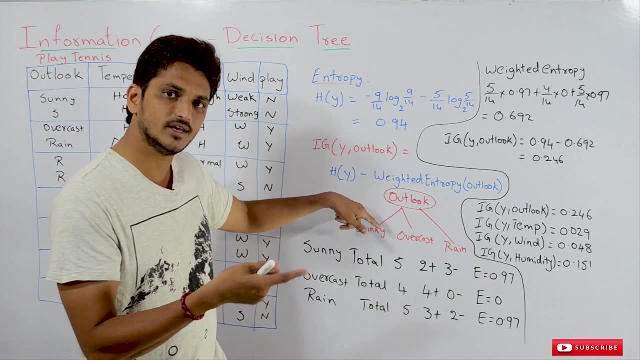 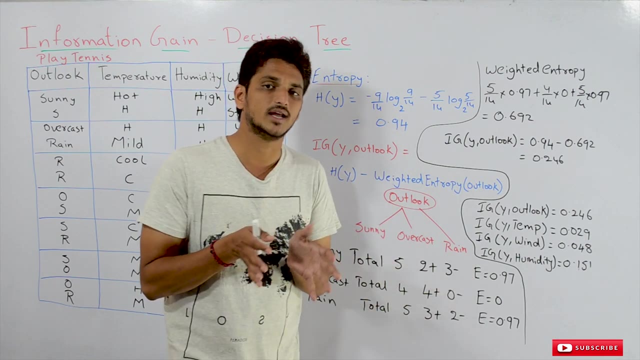 If the entropy value is maximum, we are very uncertain to do prediction. That is what we discussed. So which column we are selecting here? So the values that are having minimum of entropy values, That is, the columns we have selected. Weighted entropy value minimum. 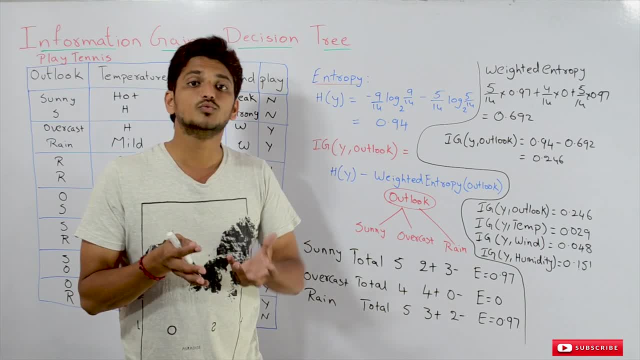 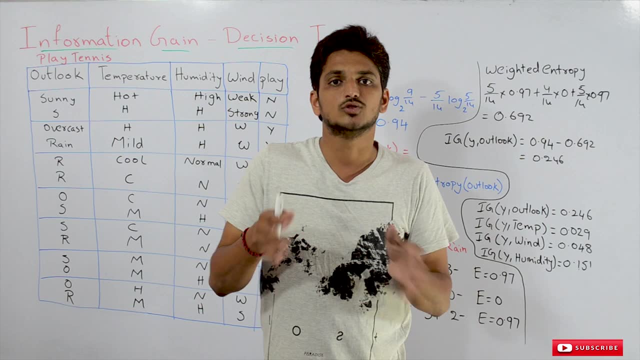 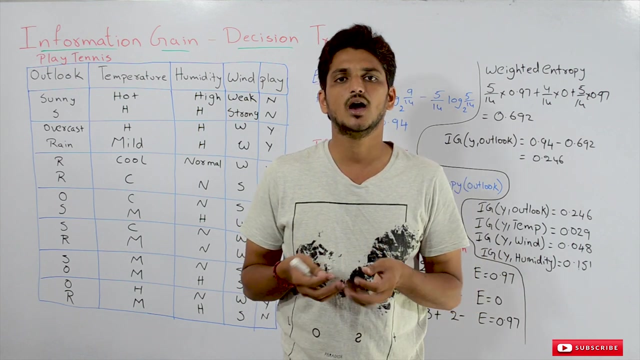 That column we are selecting Means. we are selecting the column That is helping us in doing the best prediction, That column we are selecting. So in our example, what is the best column for now? Outlook is the best column. We select it as a root node. 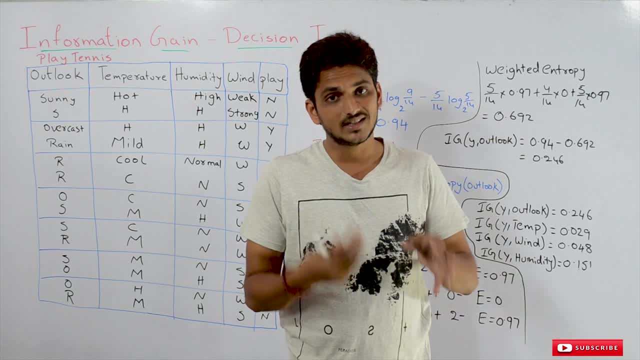 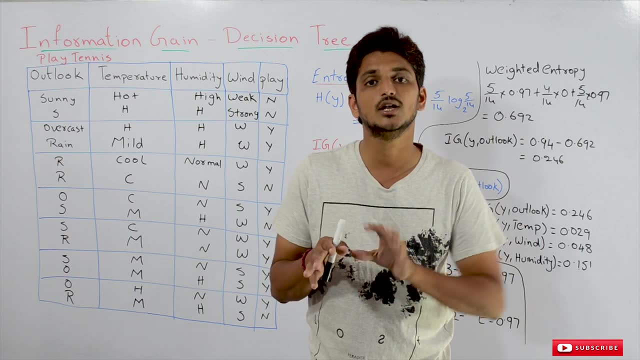 Then we have to split the decision tree and then extend the decision tree. So how to construct the decision tree using information gain- We will discuss it in our next class. Here we will understand what is information gain and how it is helping us in identifying it. 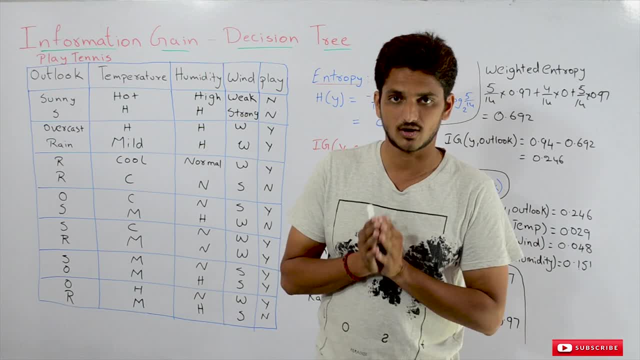 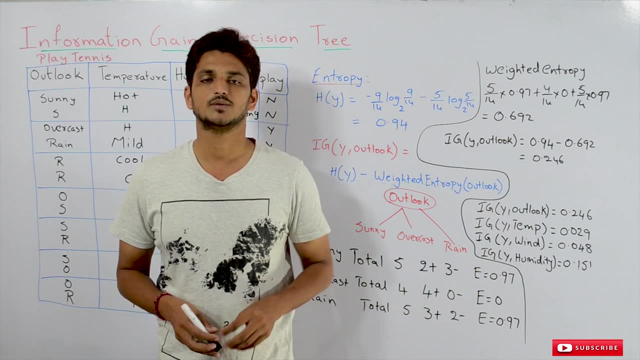 So here you see that the Że bulb is held. The relationship between the larger vector group and the larger vector group is helping us in identifying the best column. Hope you understand the concept. If you have any questions regarding the concept, please post your questions in the comment section below. 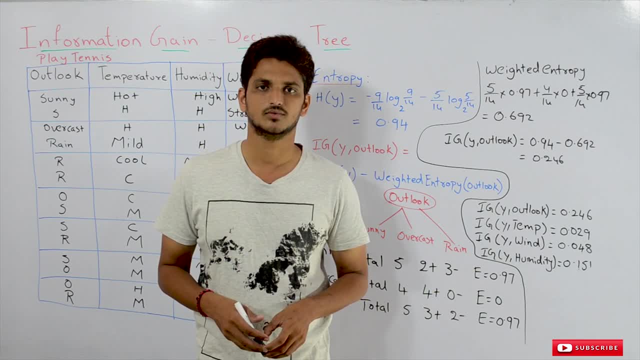 Thanks for watching. If you have not subscribed to our channel, then please subscribe and press bell icon for the latest update. Thank you.